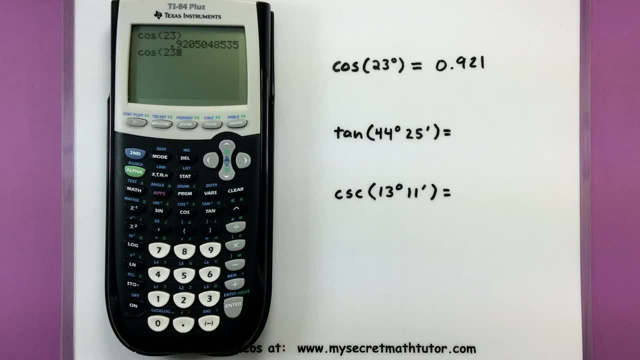 in there. I could say cosine 23 and then actually give it that little degree marker. To give it the degree marker, we have some angle options. so I can go to second and then press the angle And here you'll see those units like the degree marker, minute marker. so I can use those. 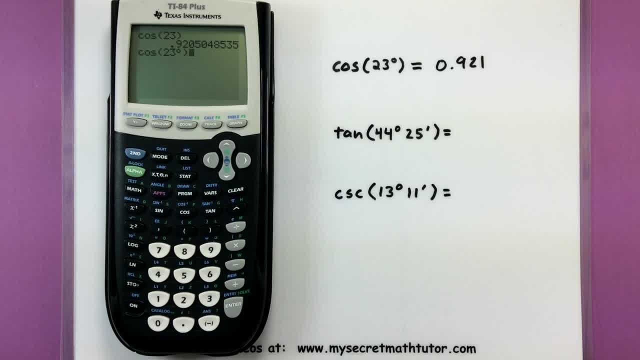 to be a little more specific. So now it's cosine of 23 degrees, and when I press enter, sure enough, I get that same answer. so nothing has really changed. Now let's go ahead and do another one, and we'll need to use that degree marker, because I have something like: 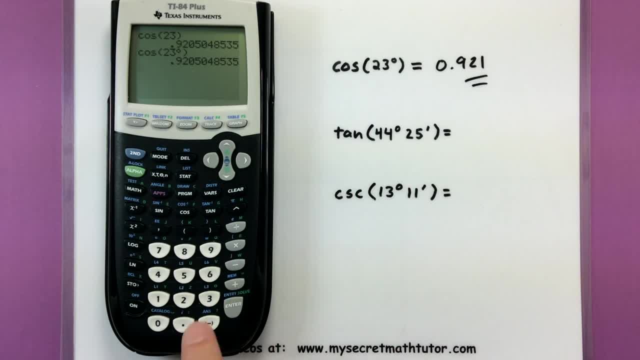 44 degrees and 25 minutes. So this one involves tangent, so I'll start off with my tangent button, I'll do 44, second angle so I can put in the degree marker, enter, and then 25, second angle and I'll put in the little. 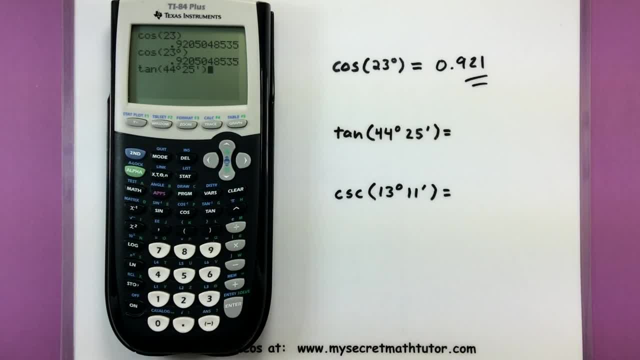 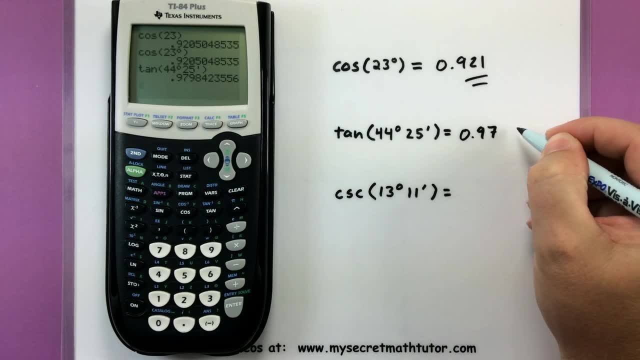 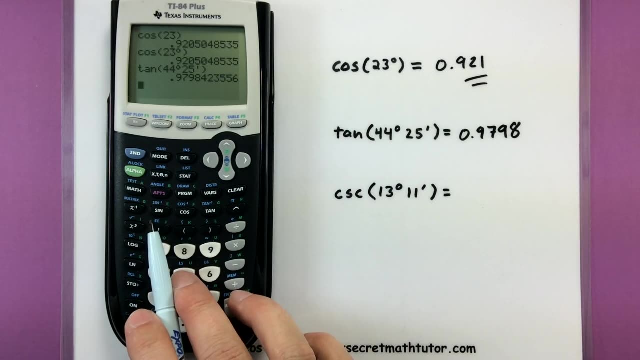 minute marker, So 44 degrees, 25 minutes. Close our parentheses and press enter, So 0.9798.. Not bad, All right. Now you'll notice on many calculators we usually only have sine, cosine and tangent And you can figure out the values of the other trigonometric functions by looking at this. So I'm going to do sine, cosine and tangent And you can figure out the values of the other trigonometric functions by looking at this. So I'm going to do sine, cosine and tangent And you can figure out the values of the other trigonometric 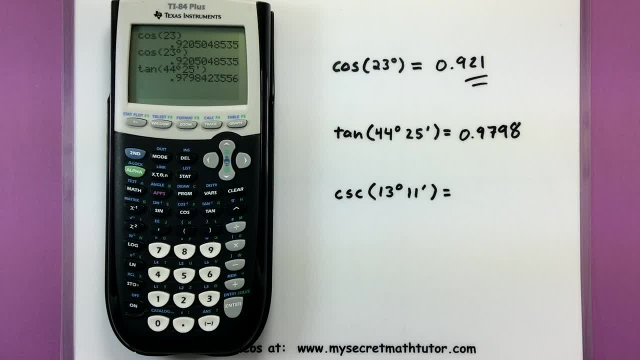 functions by looking at this. So I'm going to do sine, sine and tangent- And you can look up to my spreeder 선생- And what I can do is recognize that cosecant is the vercipical of sine. So instead I'm going to figure out what is 1 divided by sine of 13 minutes. 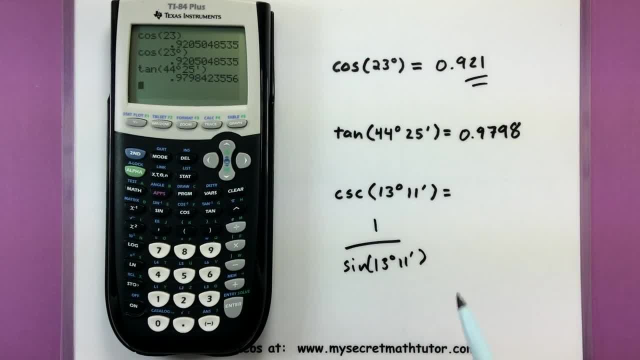 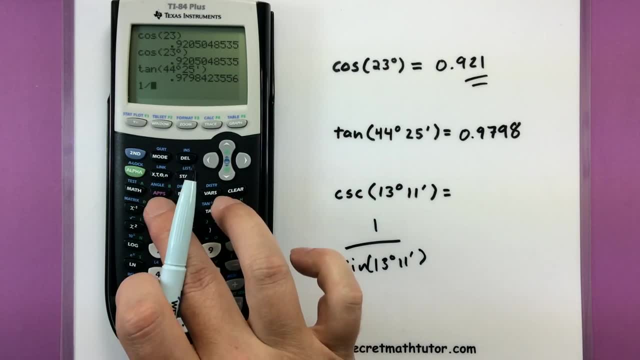 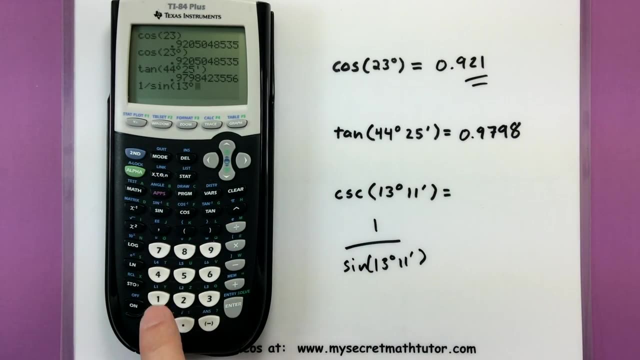 or 13 degrees, 11 minutes, And that'll give me the same value as my cosecant of 13 degrees 11 minutes. So works just as good, Right? So 1 divided by sine, squared with sign, and now let's do our 13 second angle degrees, 11 second angle minutes, close our.